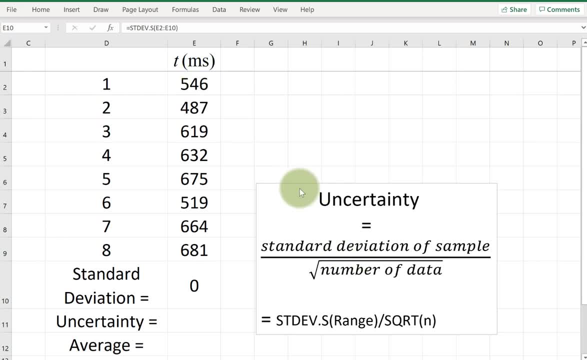 In this video, we are learning how to find uncertainty using Excel. The formula for the uncertainty is a standard deviation of the sample divided by the square root of the number of data points. The Excel function looks something like this. So let's get started. So let's type the standard deviation. 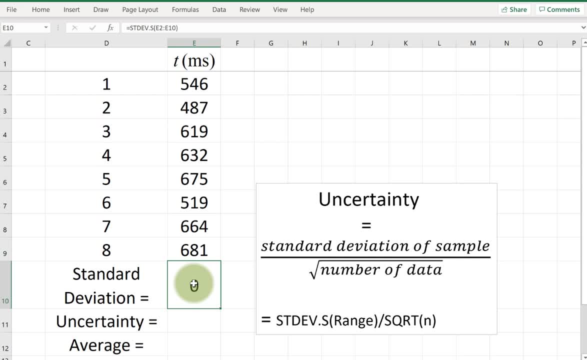 here. So before I use any formula in Excel, I need to type the equal sign and then I start typing standard deviation. and there are quite a few suggestions here. I like to use standard deviation for the sample, not the standard deviation for the population, And then I need to enter the range of the data. So in this 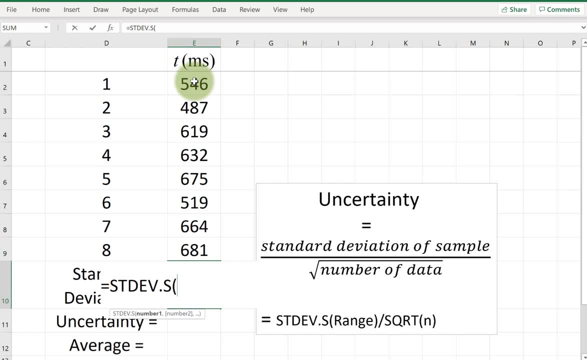 case, my data is in the cell located, for example, E2 to E9.. So I can manually type it, or I can just select the first one and then hold the shift key and the select rest one. So, as you can see, it shows you the range, And now I close the parenthesis and hit. 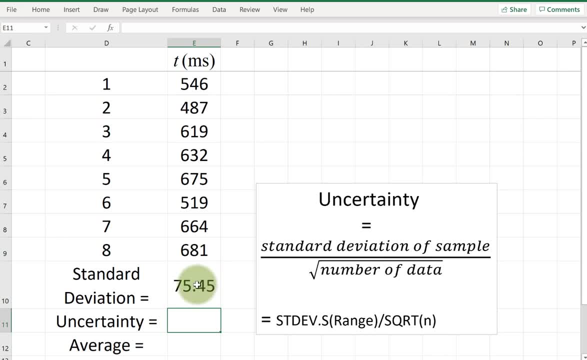 the enter sign and that gives me the standard deviation. So next step is to just find the uncertainty From that standard deviation. So that means all I need to do is I need to again type equal sign, select the standard deviation I already calculated and divide that by the square root of the number of data points. And in this: 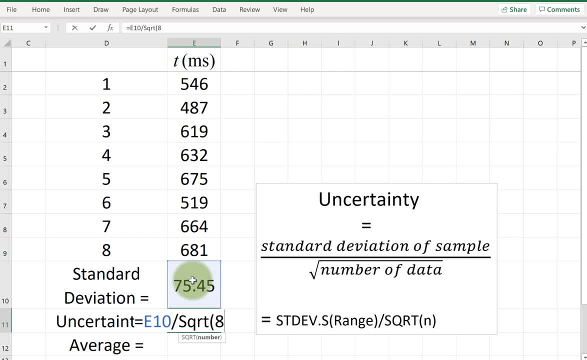 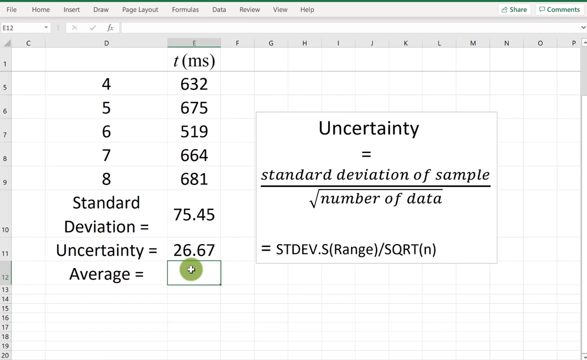 case we have 8 data, So I'm going to be using this number 8, and then close the parenthesis, hit enter and there is uncertainty. Let's also calculate the average of the data, because we're going to be using this a lot. So for this, I start by typing equal sign and then I type average or choose. 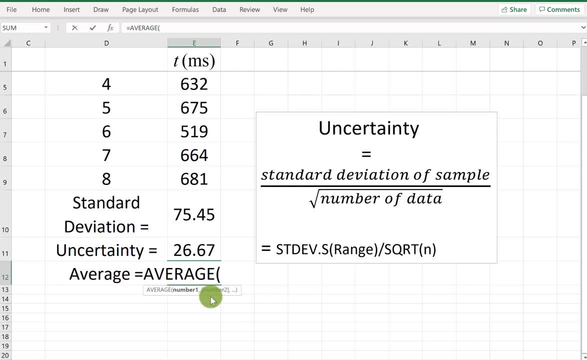 average from the list and then type the range, this time E2 to E9, and hit the close parenthesis. And then I type the average from the list and then type the range, this time E2 to E9, and hit the close parenthesis.